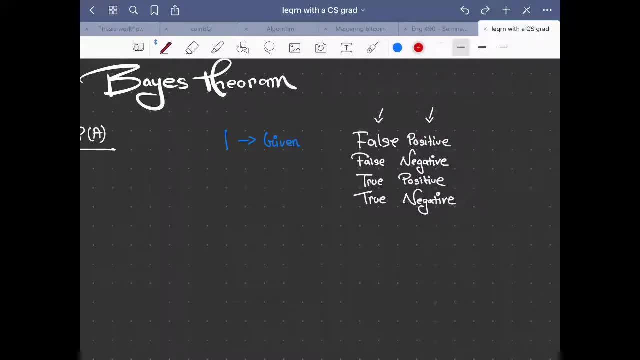 and silence the xenomorphic equation for the combination of B and B. So this is a one 매 one. test results, right? so false positive that means that you have don't have cancer, but you are tested positive. so that's never good, right? you don't have cancer, but the doctor tells you that. the reports 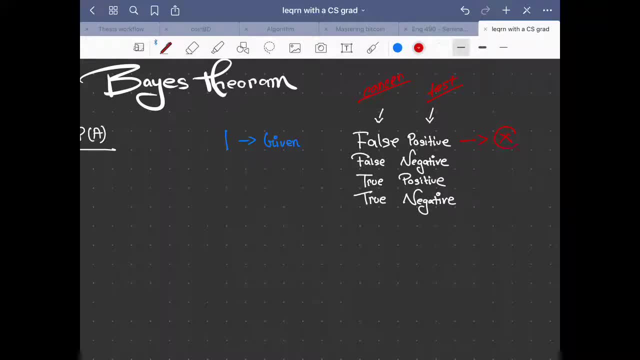 say that you have cancer. so that's never good. so false, negative, so you don't have cancer and the test results say that you don't have cancer. so this is good, this is what we want. so, and true, positive is similar. so you have cancer and uh, and the test results are also positive. so that person 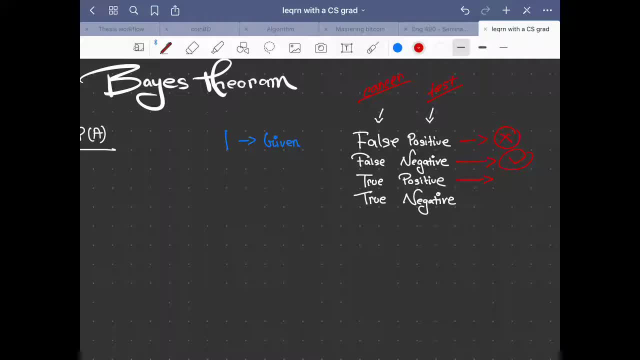 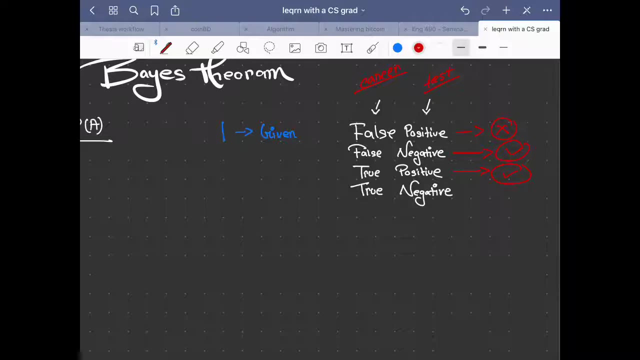 has cancer and he has been properly diagnosed with it, so, which is not good, but, uh, it's better to identify it at the early stages, right? so this is kind of what we want. and finally, you have cancer. the person has cancer and is tested negative, so this is like one of the worst things. 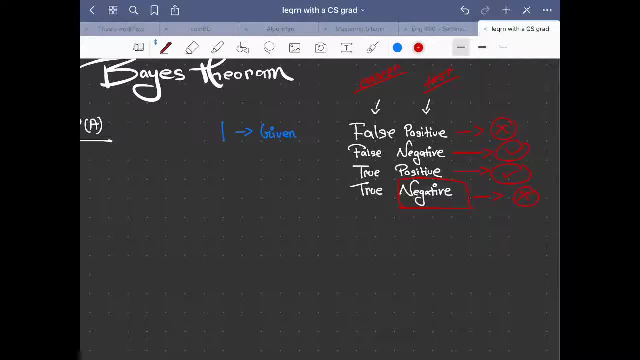 as you already have. that person already has cancer, but uh is tested negative, so you have to live with it and uh things might get worse later on. so these are the two things that we don't want in any uh situation whatsoever. so let's try to look into a question, an example, and see. 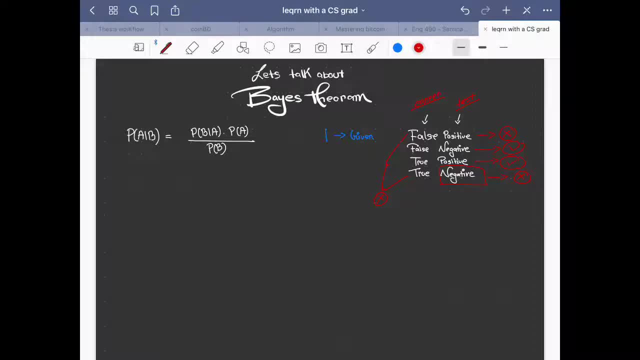 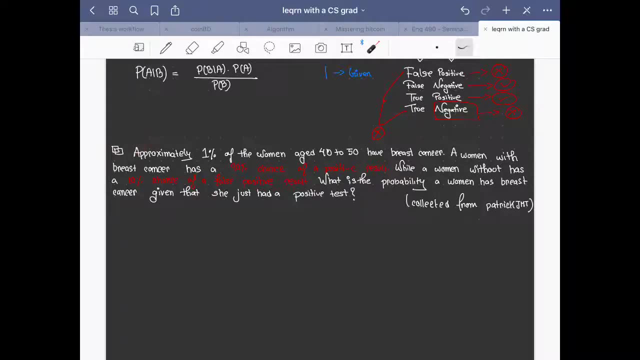 how this comes into play and how base theorem helps us to understand, uh, real life situations. so this is the question that we will be working on. so the question i collected from patrick gmt. it's a youtube channel. you can look it up- pretty good for anything mathematical related anyway. so 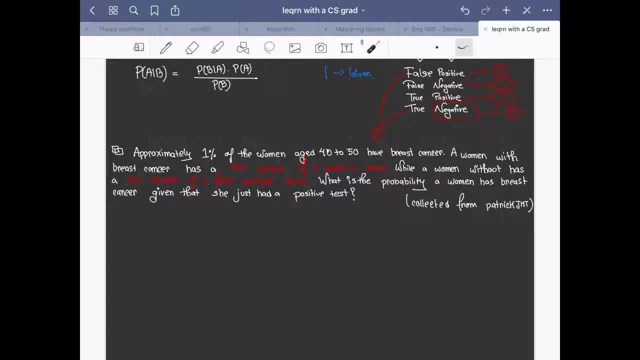 the question says approximately one percent of women age 40 to 50 have breast cancer. so there are a lot of statistics here. i don't know if they're correct or not. moving on, a woman with breast cancer has 90 chance of a positive result. so if the 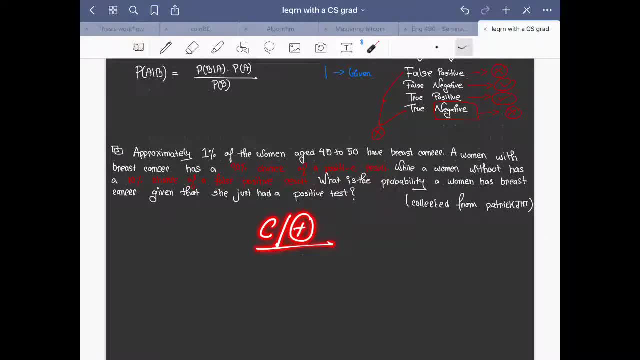 person has cancer and the test is positive. so it's. uh, there's a 90 chance of a situation being that, while a woman without has a 10 chance of a false positive result. so, uh, the woman doesn't have cancer, uh, but the results say she does, so there's a 10 chance of. 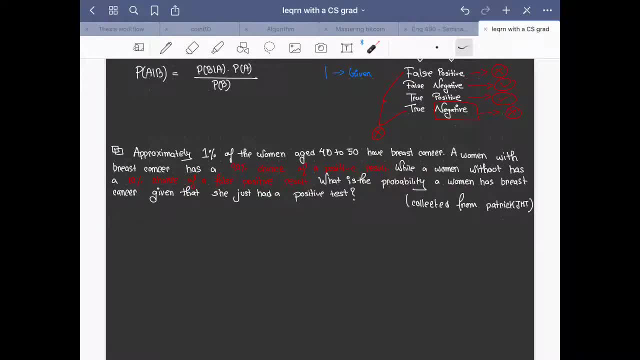 that happening? what is the probability of a woman has breast cancer, given that she had a positive test? so uh question is asking for: is that the test results are positive? however, we want to know that it is the woman. does the woman actually have cancer or not? so the the thing that we are trying to find out. 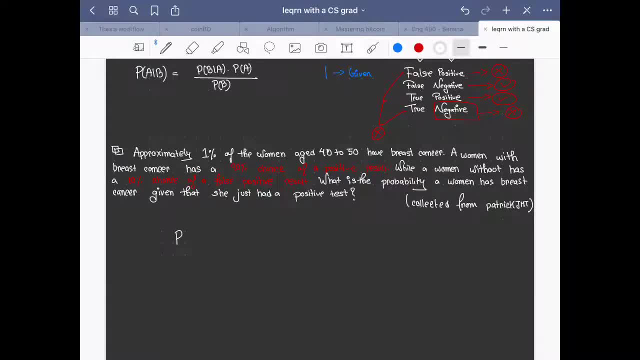 is basically this: so p the woman has cancer and she has been tested positive for it. so this is what we are looking for, right? uh, so, according to base them, so the situation would be: so she is tested positive for cancer, given that she actually has cancer, into the probability of a woman having cancer divided by the probability of the test being 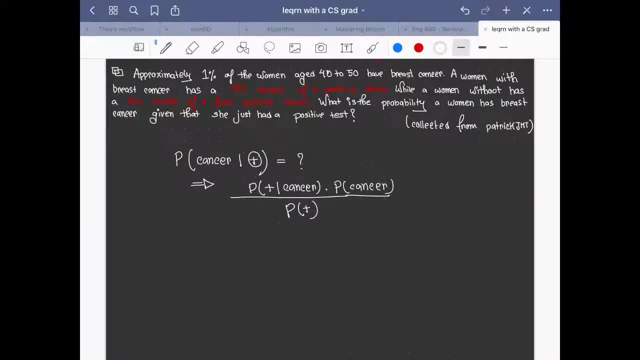 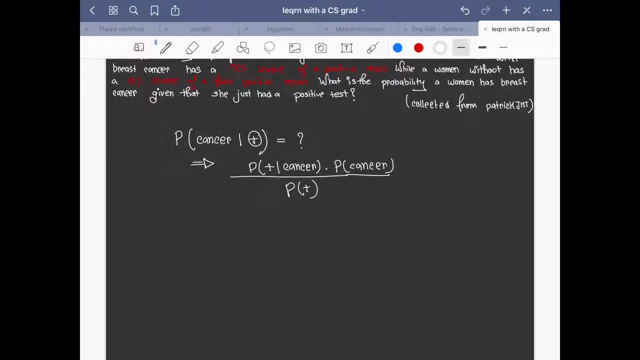 positive. so, uh, uh, in your classes or in the examples, you might see that they just put values and try to calculate it. however, i'm going to follow a tree structure, which is like much easier to understand what's happening. so, so, this is the main situation. this is like our starting place from this. 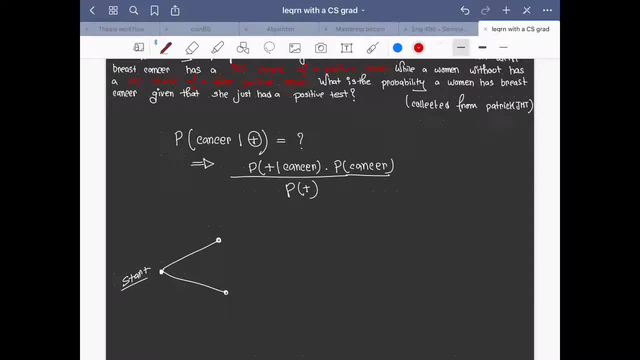 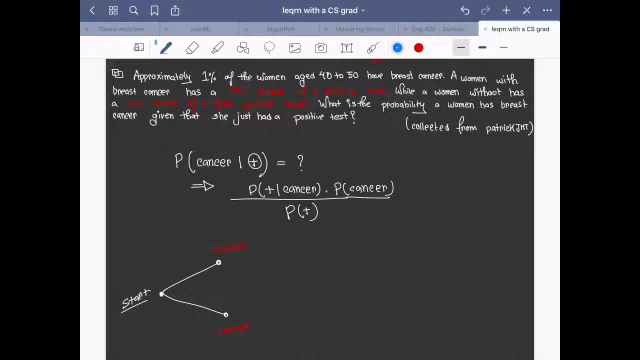 we would have two situations. so one where the person has cancer, and this is the person doesn't have cancer, right? so what's the probability for that? so this says there's 1 percent chance of women age 40 to 50 have cancer. so this is 0.01, uh, 0.01, a chance of a person having 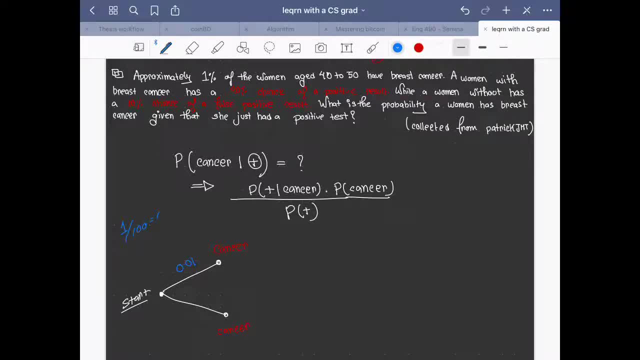 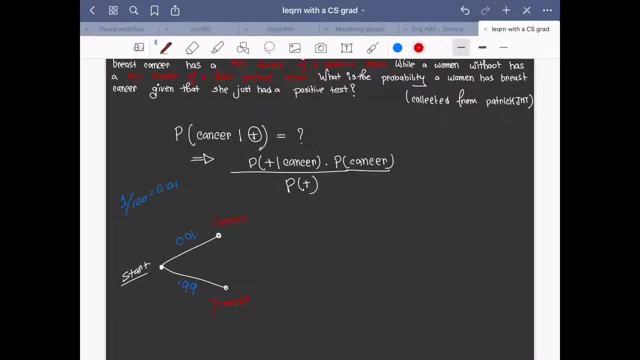 cancer. so it's 1 percent. so 1 divided by 100 is 3.01. that's why uh written that, and there's a 99 percent chance that the woman might have cancer. this is an odd sign, so uh, moving on. so what can happen from here? so there will be two situations. 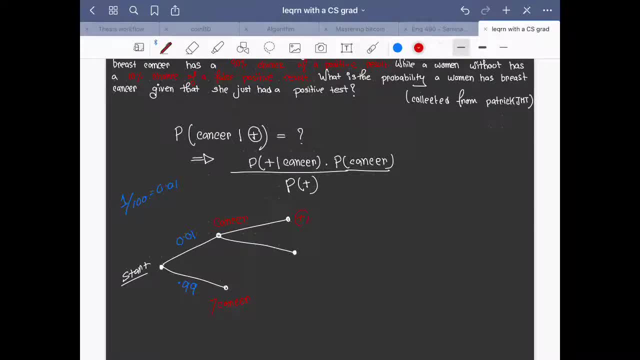 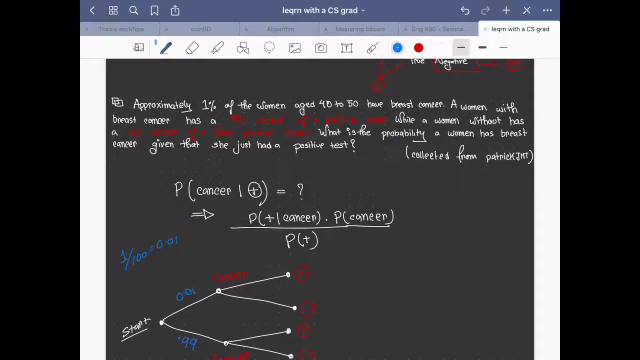 so the situation is that the person is tested positive and the person is tested negative and similarly, from this place we would also have two situations: the person is tested positive and the person is tested negative. so what are the values here? so, according to the question, so a woman with breast cancer has ninety percent chance of 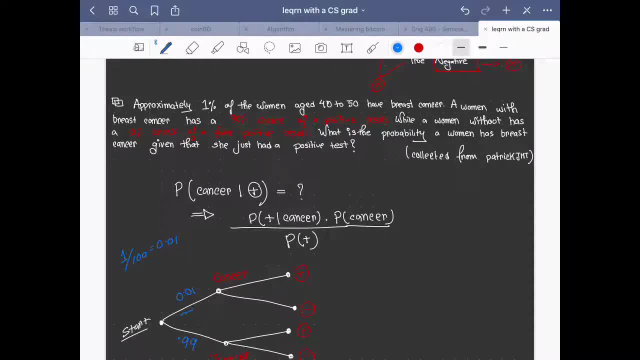 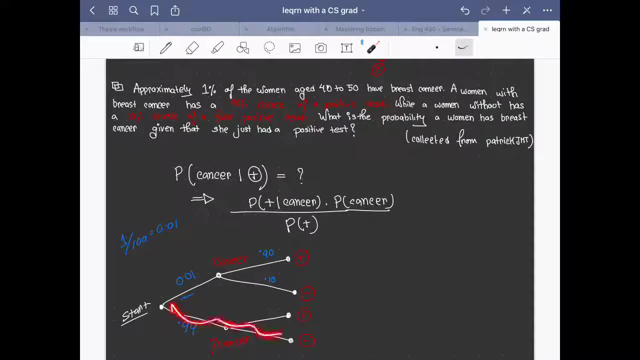 a positive result. so this portion, this is basically the person has cancer and there's a ninety percent chance of them having this, so 0.90 and this would be 0.10, and while a woman without. so we would be looking into this portion here. uh, without. 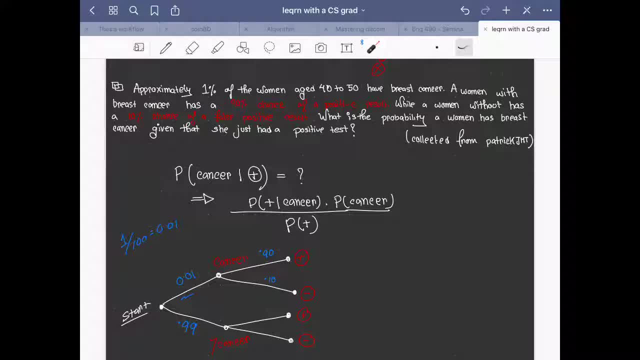 has a 10 chance of a false positive. so this means that this portion means that the woman doesn't have cancer, so but it's still tested positive. so would be one percent and one zero. so point one: zero, and this would be point nine: zero. so let's try to. 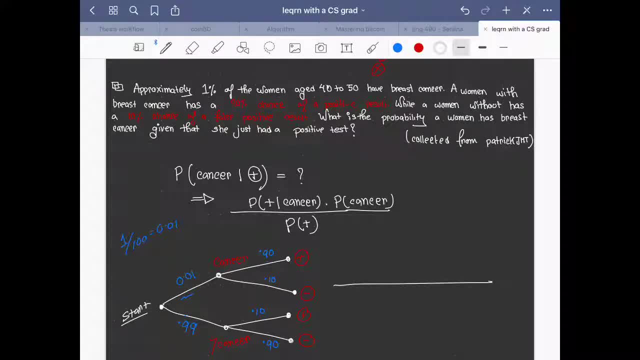 find out what would actually happen. so you put values up in the equation here you would get the answer that we're looking for. so first portion says that the woman has cancer, is stasis positive and actually has cancer. so we'd be looking into this branch. so the person? so let's try to highlight this, this is: 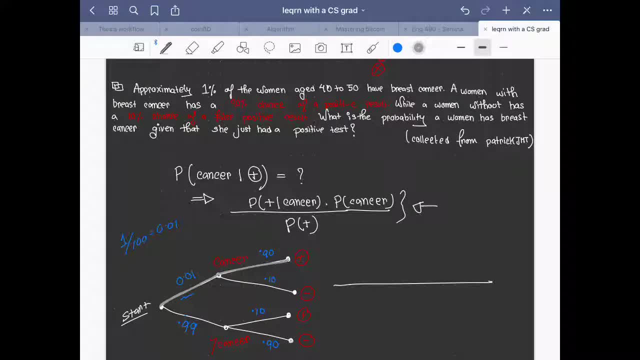 what you're looking for. the person does have cancer and stasis positive. so let's write the equation like: write the values down. so it would be point nine, zero, into point zero, point one, and below that we have the probability of the results being positive. so this: 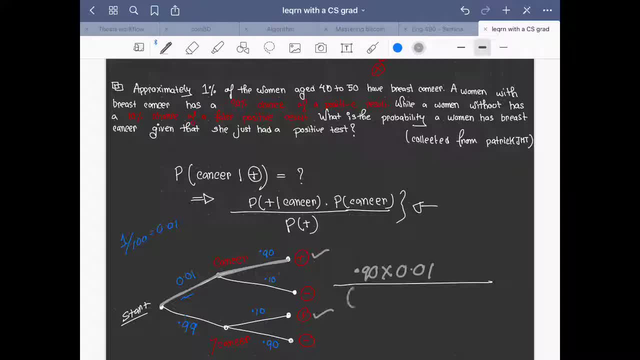 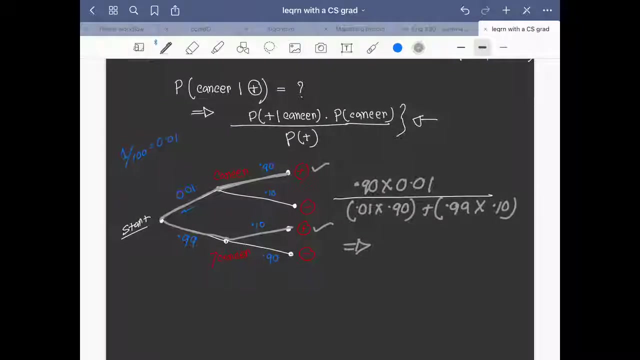 would be this situation and this one. so that's right: 10 down, 10 down, 1, 2, 1 would be 0.01 in to, and i do the same thing that we have written above, plus and this case, so in two points work. so the result would be so this is the.